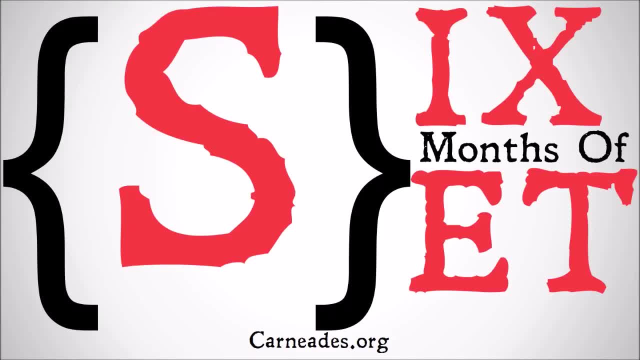 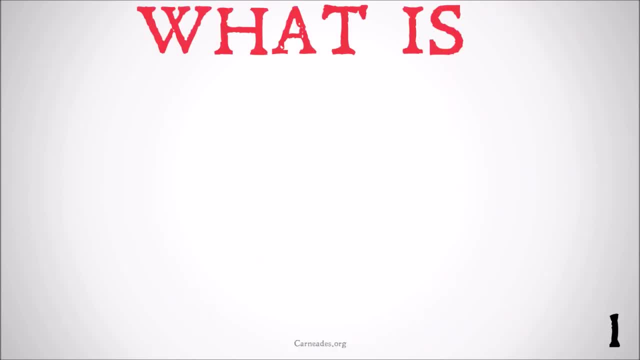 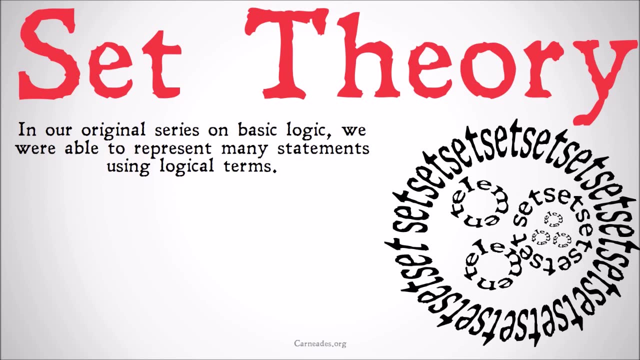 Welcome back to Cardinalityorg. Today we're going to be continuing our series- six months of set theory and higher order logic. This is our logic 301 series. In this video we're going to be looking at what is set theory Now. in the original series we did on basic logic, we were able to represent many statements using logical terms. We could say Socrates is a man. We could say no, men are immortal. We could say Socrates is not immortal Using letters to stand. 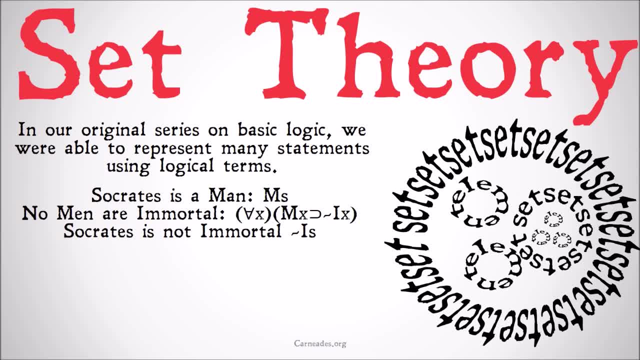 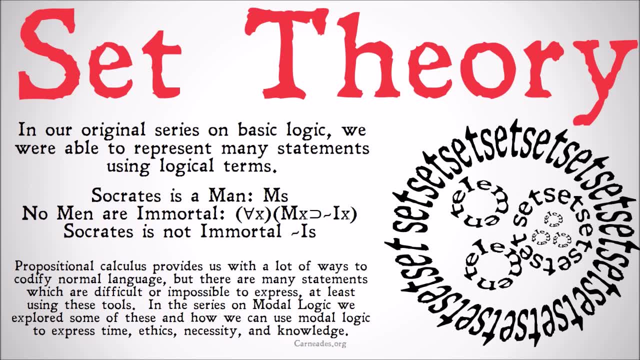 in for predicates and subjects and then using the underlying logic to show the relationships between those predicates and subjects. Propositional calculus provides us with a lot of ways to codify normal language, But there are many statements which are difficult or even impossible to express, at least using these tools. In the series on modal logic, we explored some of these and how we can use modal logic to express things like time, ethics, necessity and knowledge. 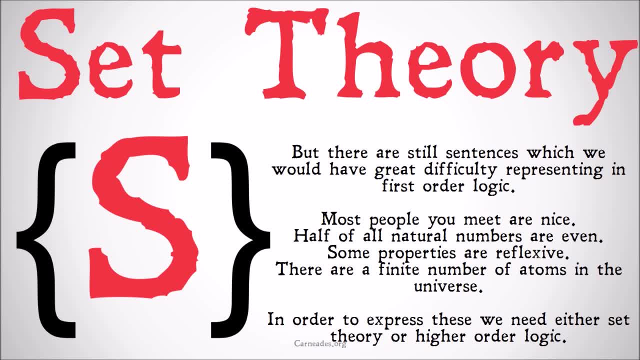 There's still a lot of sentences which we would have great difficulty representing in first order logic, Such as: most people you meet are nice. The idea of most is something that's hard to express. That more than half quantity of the people you meet is something weird that we don't really have the language to express. yet Half of all natural numbers are even. This is tough because we're talking about an infinite set of things, So we can't have an infinite set of things. 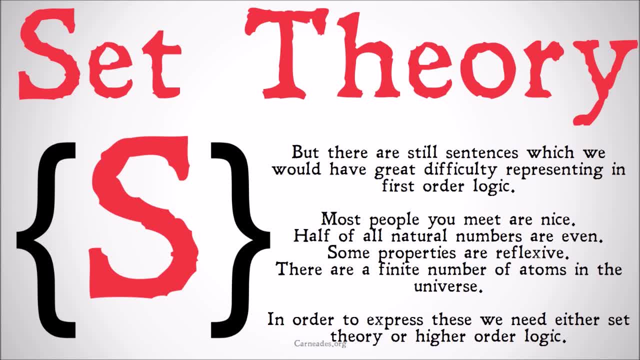 notion of an infinitely long proposition, at least not yet in important way. we understand in single, in in first order logic, Some properties of a reflexive. talking about properties of properties is something that's difficult. We've kind of fudged it a little bit in first order logic so far. But 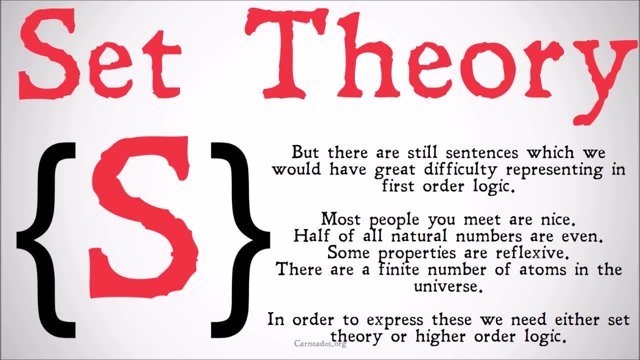 you really need something like higher order logic to do it, and there are a finite number of atoms in the universe- ones again talk about the difference between finite and infinity- is going to take something like set theory or higher order logic to do it. In order to express these, we need either: 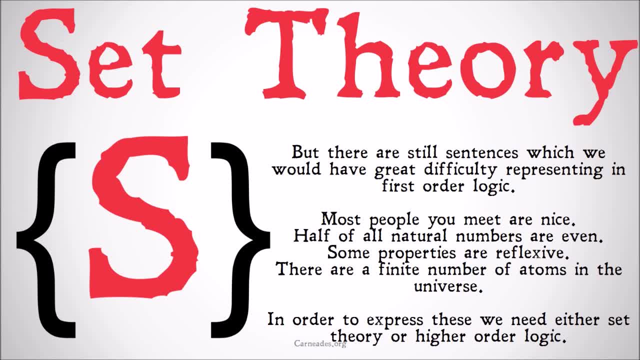 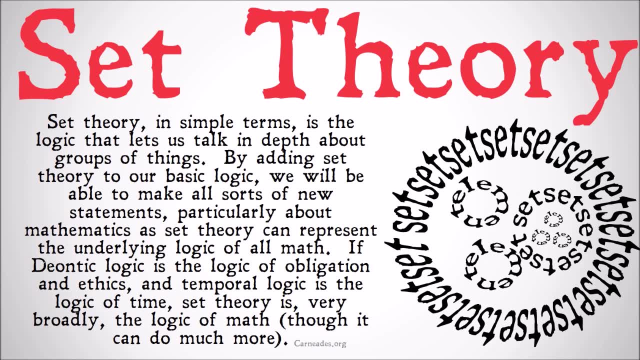 something like set theory or something like higher order logic or some combination of both. So set theory, in simple terms, is the logic that lets us talk in depth about groups of things. By adding set theory to our basic logic, we will be able to make all sorts of new statements.